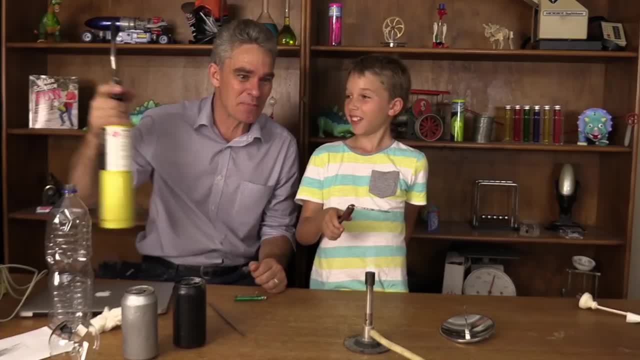 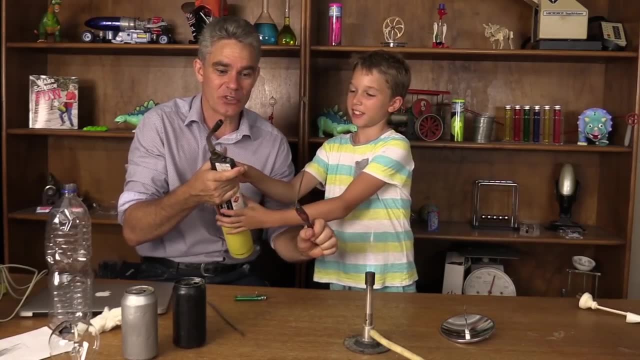 I'm going to get the powerful flame out. Are we ready, Sam? Yeah, This is the powerful flame, And so I'm going to heat this nail up with the powerful flame. Oh, Sam wants to do it. Okay, Sam's going to heat it up. 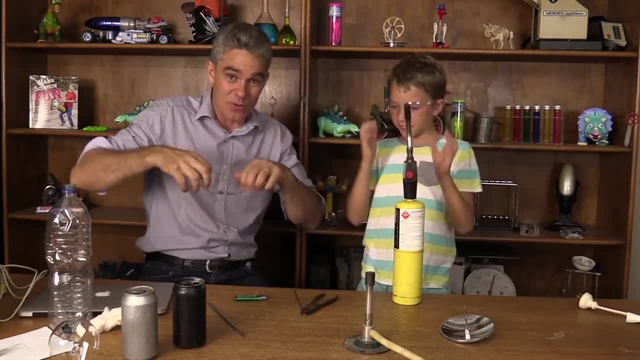 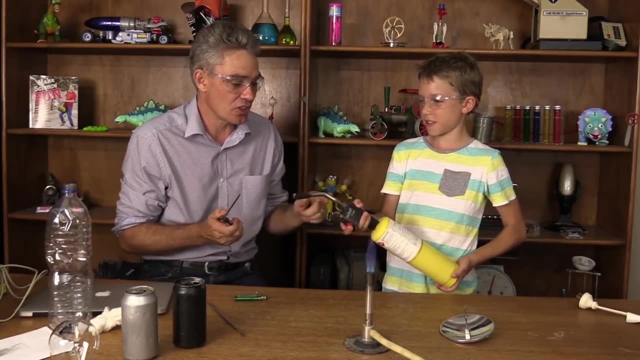 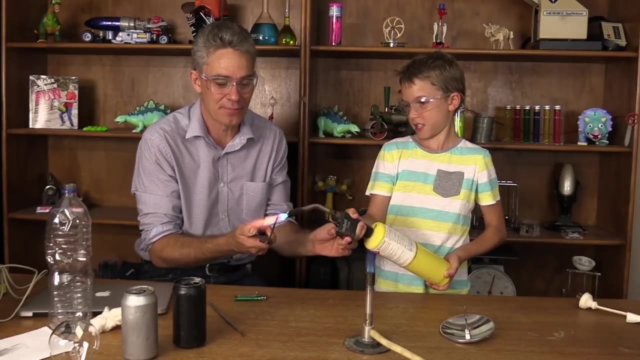 We better put on our safety glasses first. Keep our eyes safe. And, Sam, okay, you have to make sure you don't point that at anybody. Okay, So you turn that flame off, Click. Oh, look at this. Oh, look at that fire. 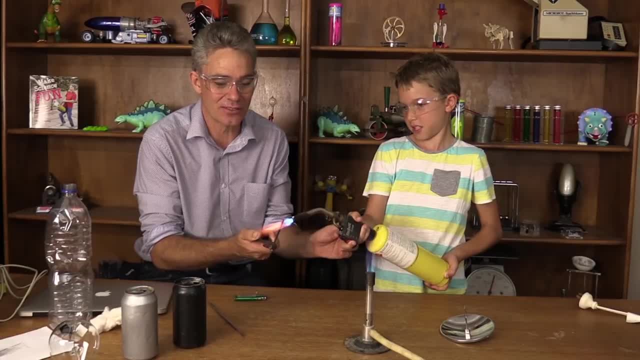 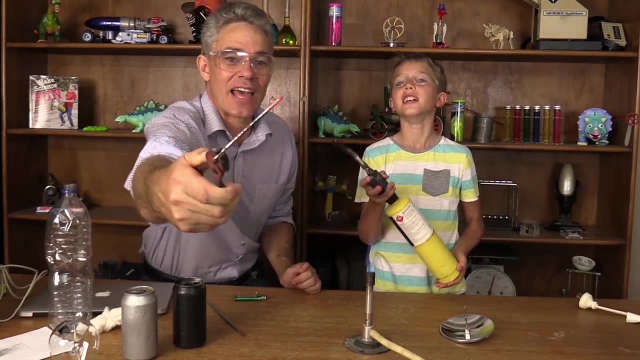 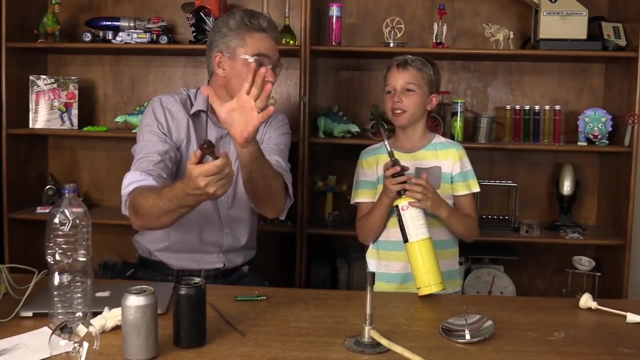 Oh, it's heating up the nail. Look at that. The nail is glowing red. Wow, look at that. Look at that red nail glowing. And do you know what I can feel? the heat from here. The heat from that red, hot nail is travelling at the speed of light and warming up my hand. 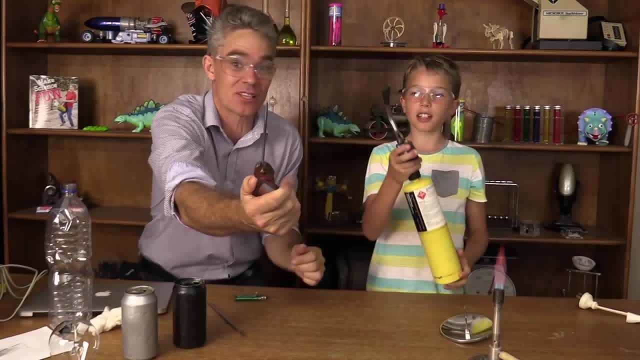 Let's do it again, Sam. We'll do it closer to the camera this time so that the kids can see it even better. Quick, Look at that. When it starts glowing, it starts a mini radiation, And this is thermal radiation or heat radiation. 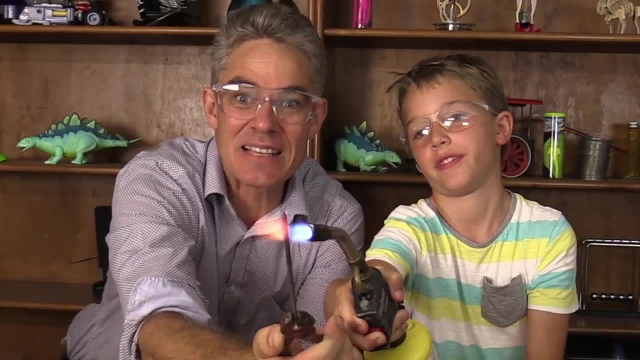 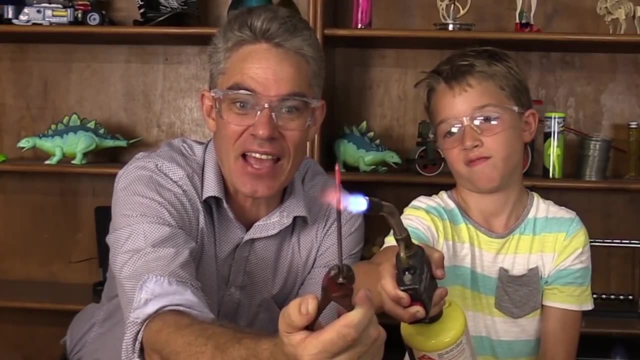 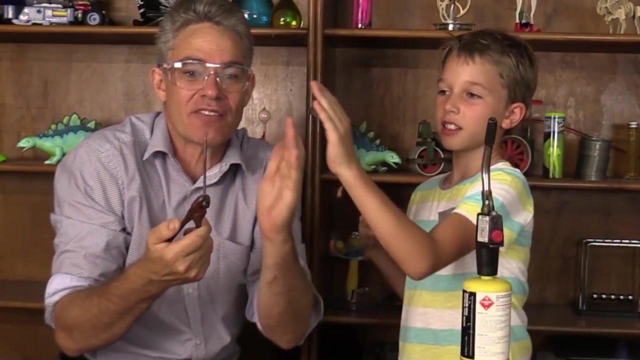 And that heat radiation is travelling to you at the speed of light. Oh, you can feel that heat travelling at the speed of light. You can feel it on the side of your hand, can't you? Yeah, Okay, Heat it up. 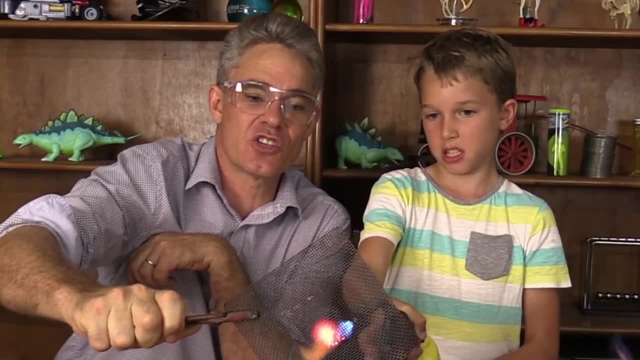 And when it glows orange, it's going to transfer the heat via radiation And Sam and I are going to be able to feel that heat. You can turn the fire off now, Sam, But we can feel the heat via radiation. And now the orange is gone. 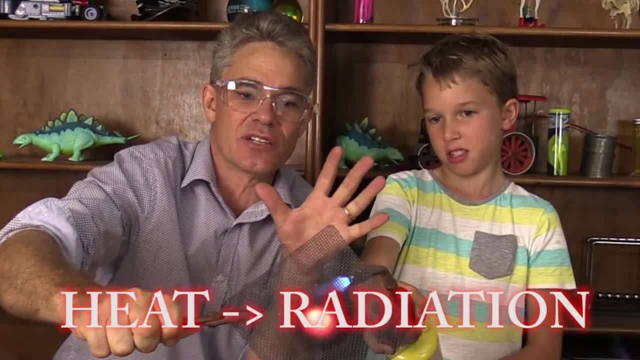 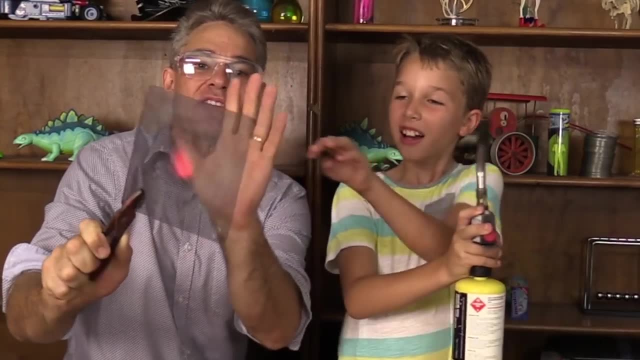 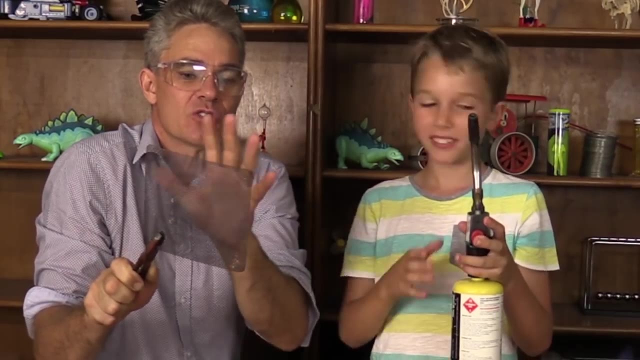 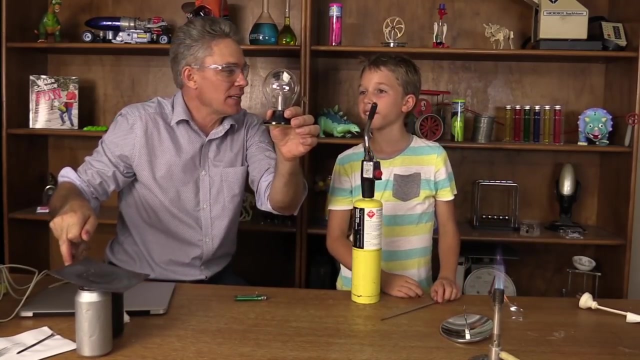 And the orange is gone as it cools off. because it cools off? because it's giving out the heat. Sam, let's go outside and have a look at the radiometer outside. Let's put our hands together and go out there Ready. 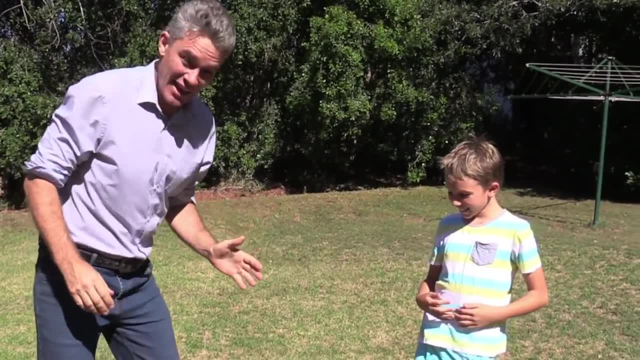 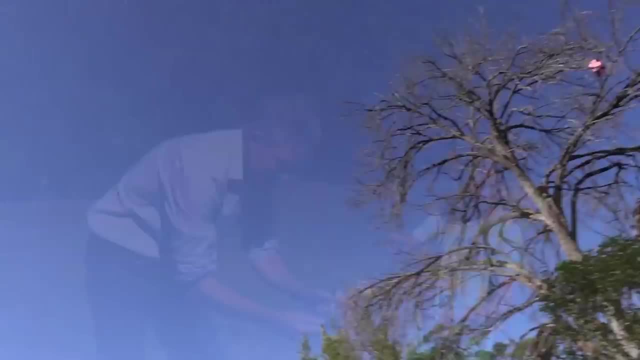 Set. Woohoo, Oh, here we are, outside, Sam, And we're in the sunshine, The radiation from the sun. it's taken eight minutes to reach us. This is called a radiometer. What Yeah, What Okay. 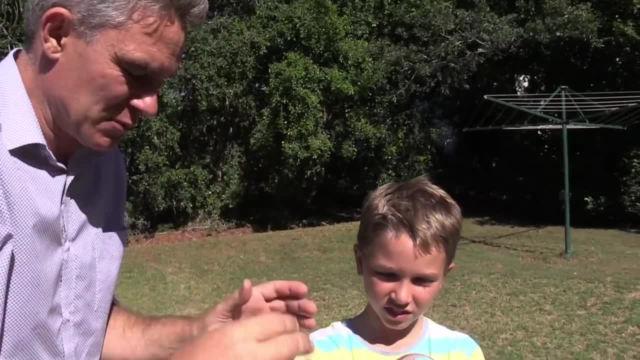 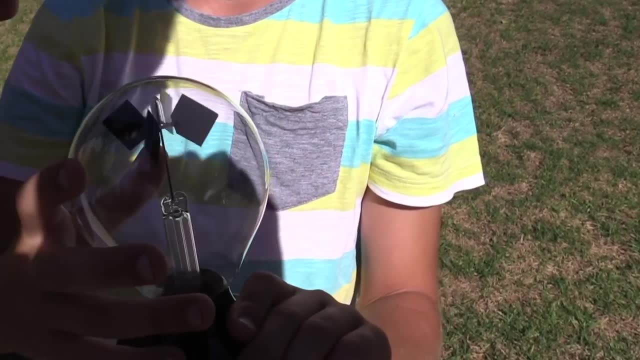 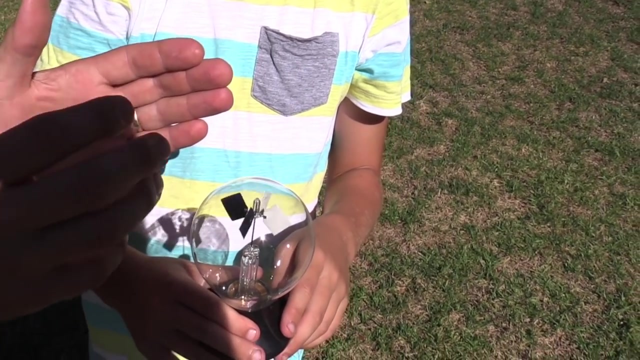 Come up close. Come up close. The radiation is blowing. The radiation is passing through the glass. The radiation is passing through the glass And it's heating up the black side of the little spinner. And as the black side heats up, it sort of ejects little air-hot molecules, causing it. 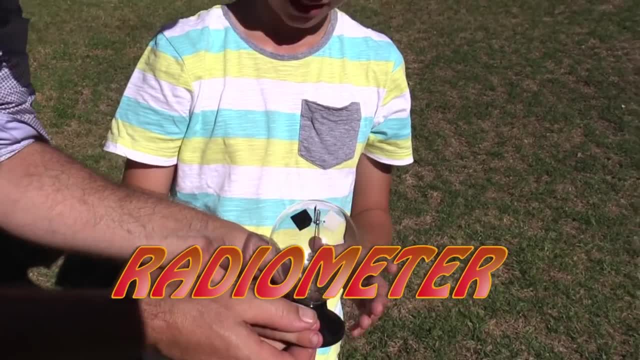 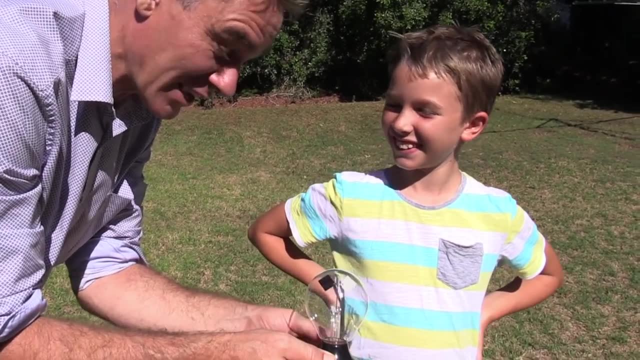 to spin in the sun. This thing's called a radiometer. It sort of shows you when there's some radiation. Look at that spin. What's it called Sam Radiation? Yeah, radiation. And what's this machine called A radiometer? 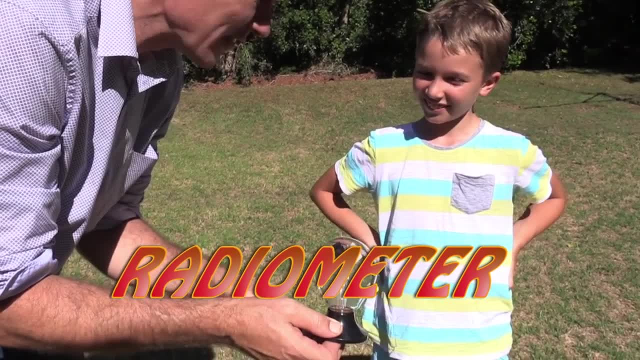 Radiometer, Radiometer, Look at that. The radiation from the sun is causing it to spin, And the radiation can actually go through the glass. Look at that. Hey, is that good? Yes, Yeah, Oh, that was a fun adventure outside, wasn't it, Sam, where we learned about the radiometer. 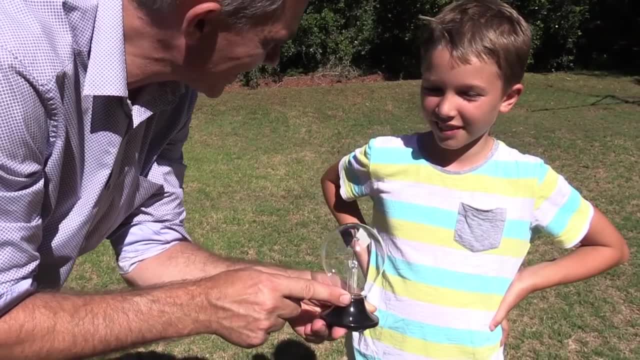 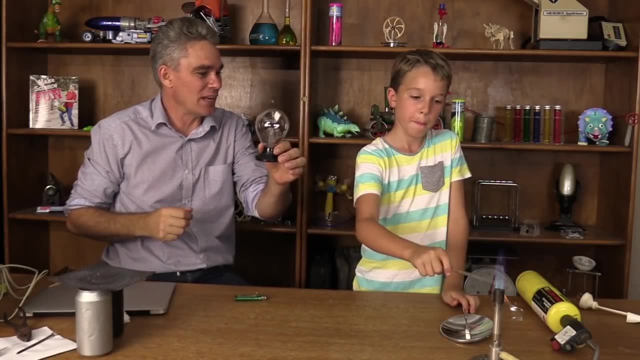 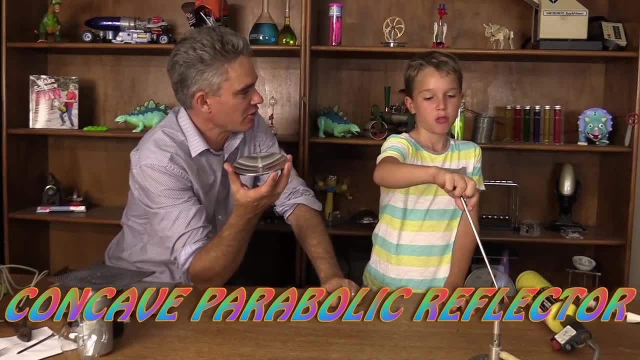 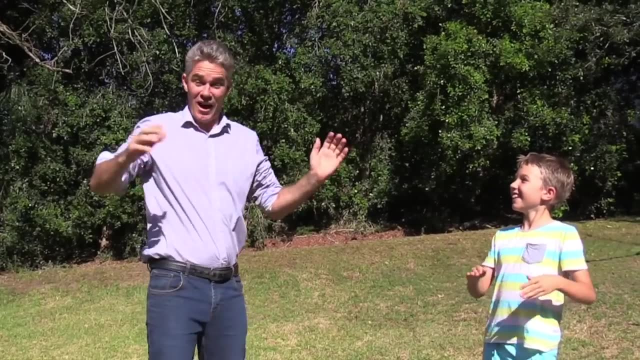 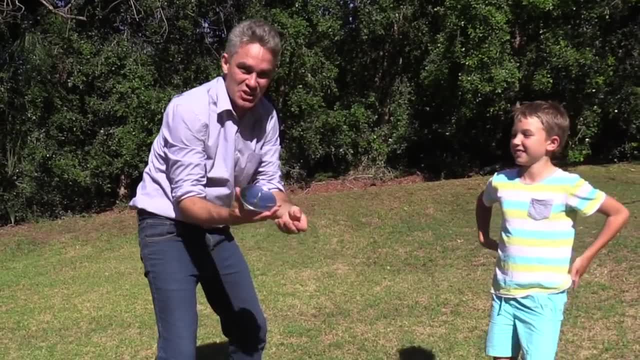 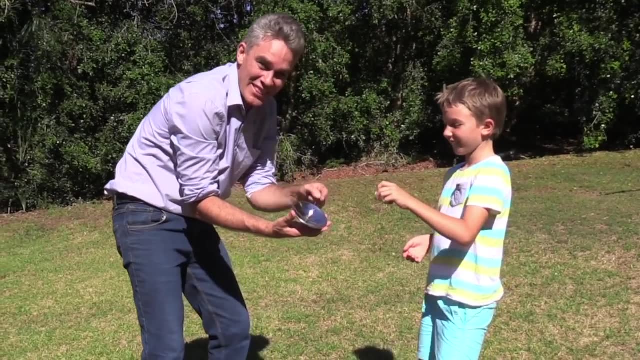 Here we are at the sun again, Sam. Oh, I've got this special concave reflecting bit And I'm going to put. Sam, you want to put the marshmallow right there at the point of focus. Put that, Yeah, that's it. 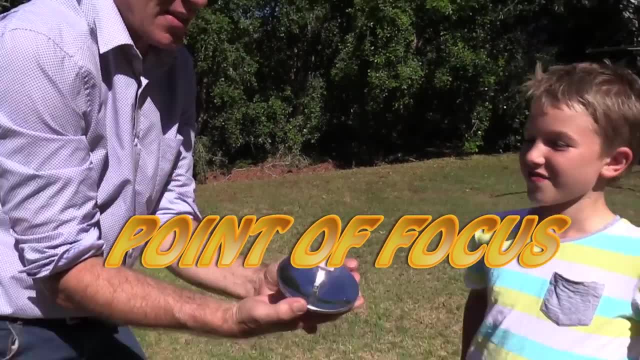 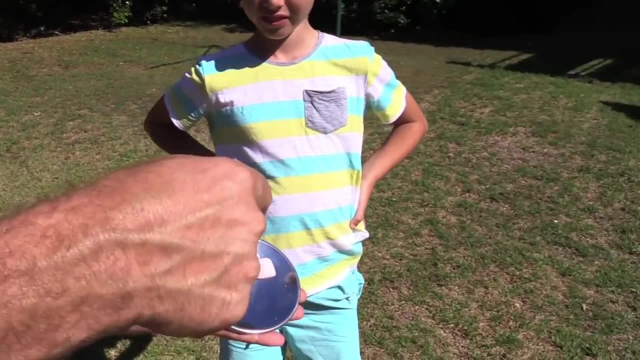 Put the marshmallow at the point of focus and have a look at this. We're going to cook the marshmallow in the heat of the sun. The sunlight is reflecting off the concave, off the concave fish, and it's hitting the marshmallow. 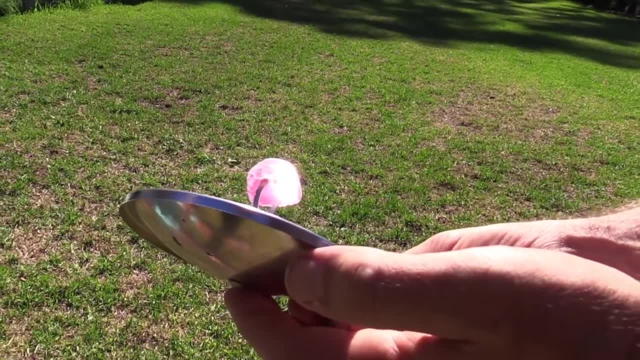 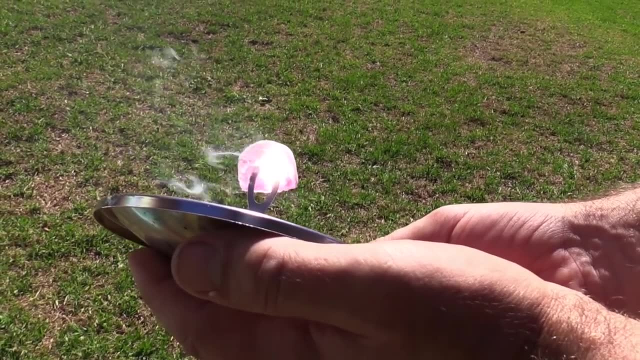 Look at that. can you smell it? Yes, What's it smell like Marshmallow. That's marshmallow. Whoa, How does that, eh? Do you wanna pull that off? Mm-hmm, And you can eat it. 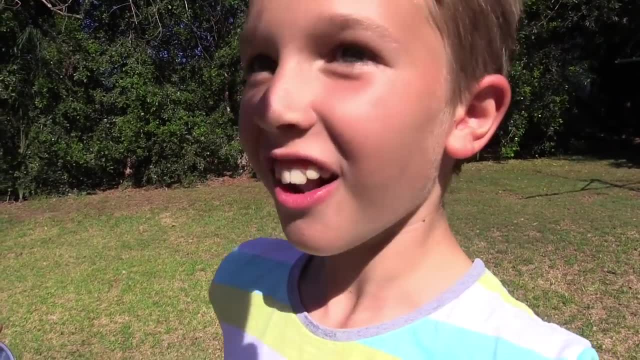 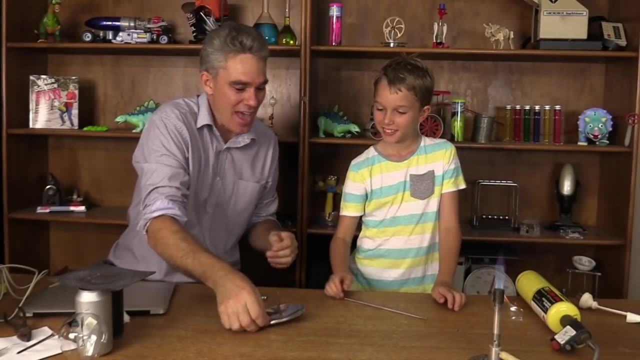 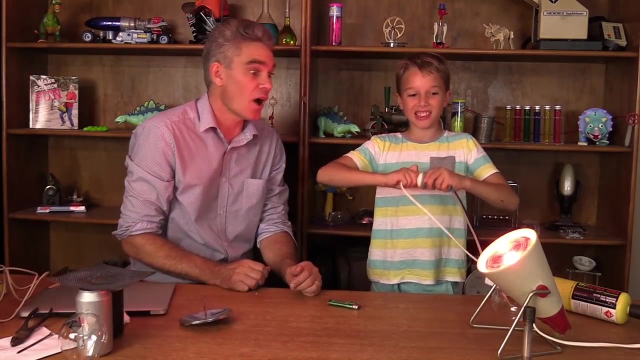 Eh, What's it like, Mm? Is it nice, Is it yummy? Mm-hmm Whoo. Oh, how good was that Exploring cooking marshmallows with the sun? Sam's gonna turn on the infrared light. 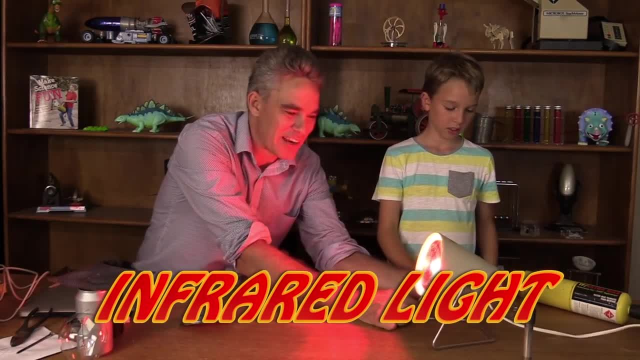 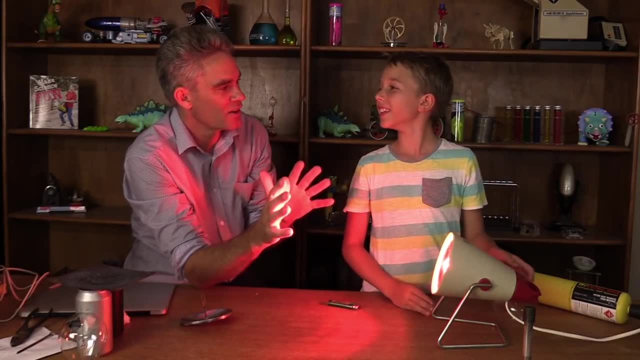 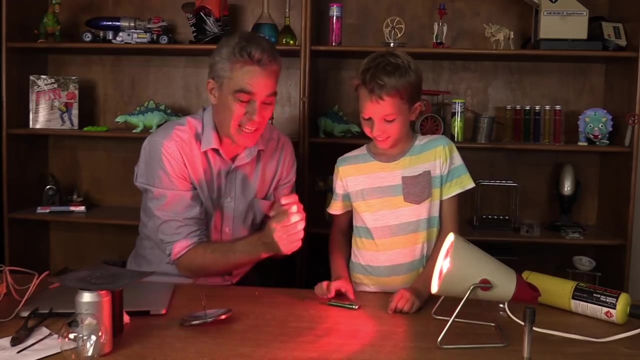 Oh, look at that, This is an infrared light. Oh. heat transfer by Heat transfer by No, By Ruh, ruh, ruh, ruh. Ray Radiation, Radiation. heat transfer by radiation Oh. 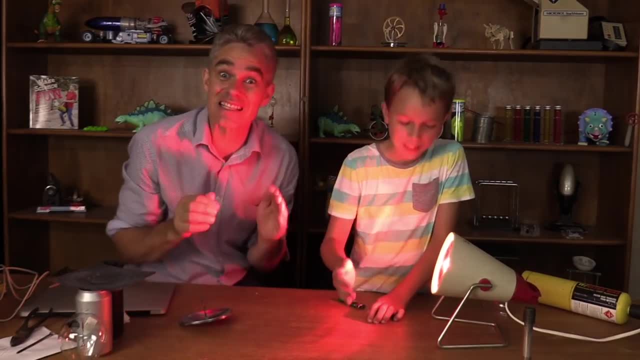 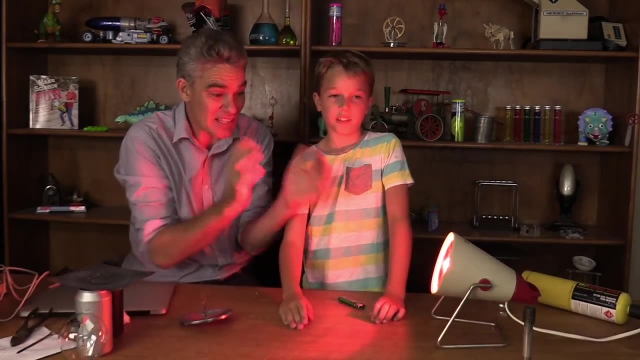 How quickly does it travel, do you think, Sam? Very fast, Very fast, At the speed of light: 300,000 kilometers per second. 300,000 kilometers per second, That's how quickly it comes. If this was the sun, well then, in one second. 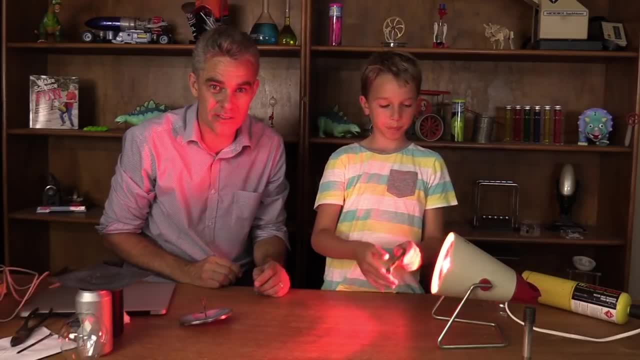 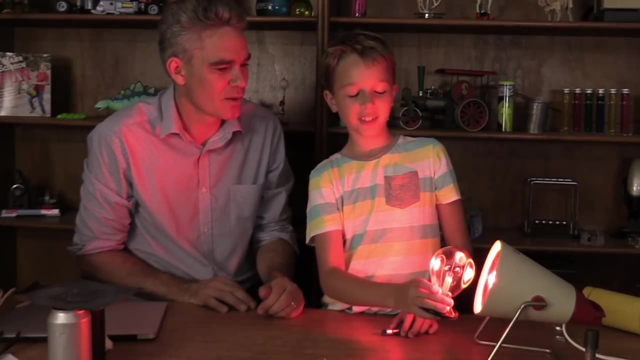 the light would travel 300,000 kilometers. That's a long way. Ah, And what have you put in front of the infrared light, Sam The um? What's this device called Radiometer, Radiometer, Radiometer. 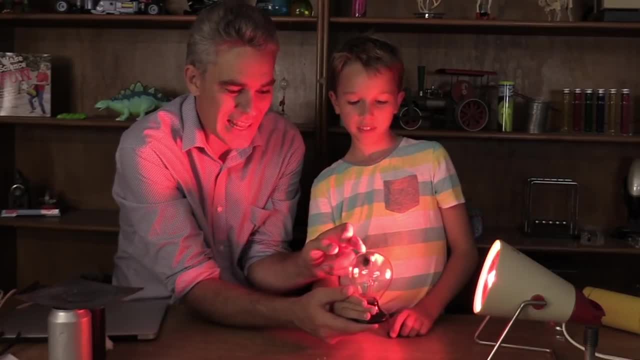 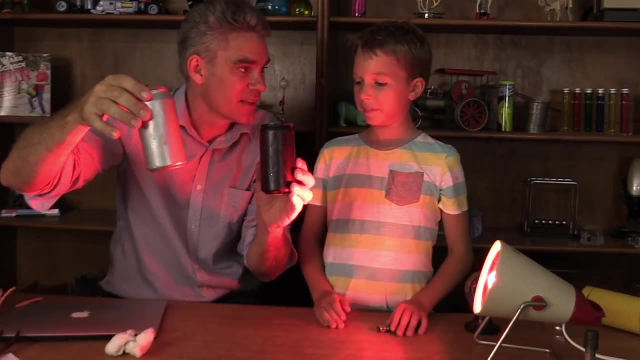 And the infrared light is going through the glass and it's heating up the little windmill and it's causing the little windmill to spin. And I've got a silver can and a black can. Now which one do you think will heat up the quickest if we put it in front of the infrared? 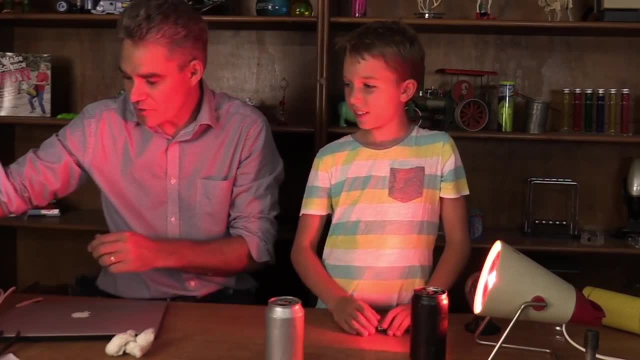 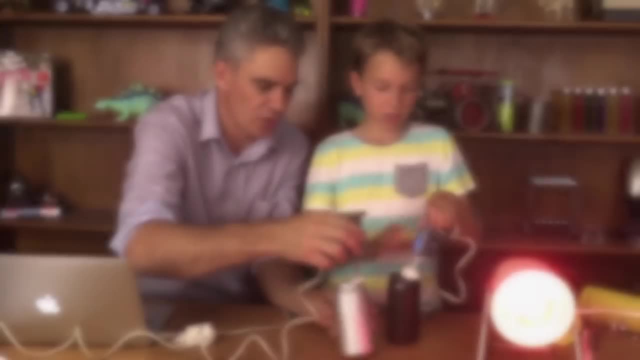 light, Black, Black, you think: Okay, So I've got some special equipment here. Can you put one of these temperature probes in to one? Put the light On them both. Putting the light on them both, You think yours is winning. 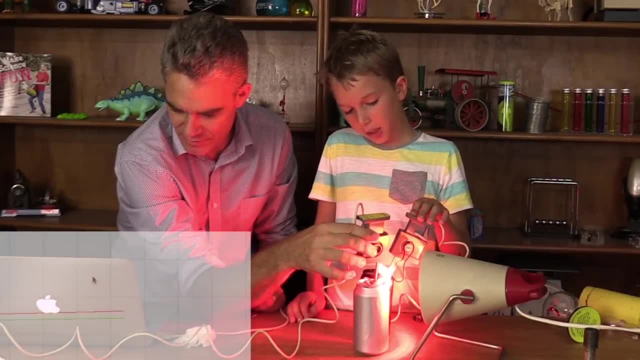 Because mine's red, Yours is the red one And you think the red one's going up more quickly, do you? Can you feel the difference, Sam? One's a black can and one's a silver can. Which one is heating up the most by the radiation? 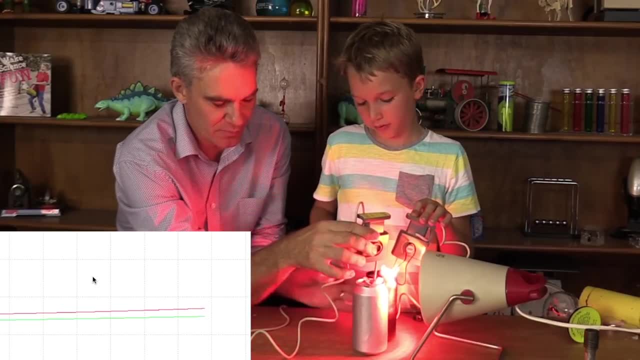 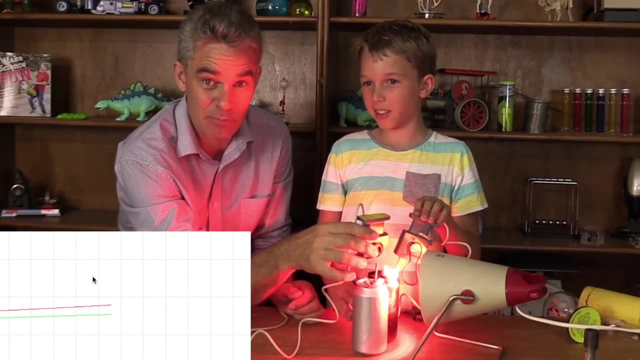 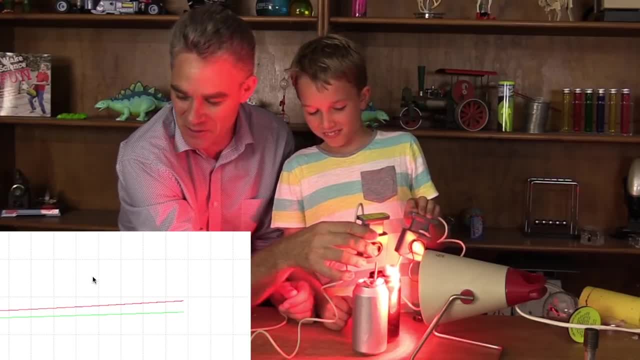 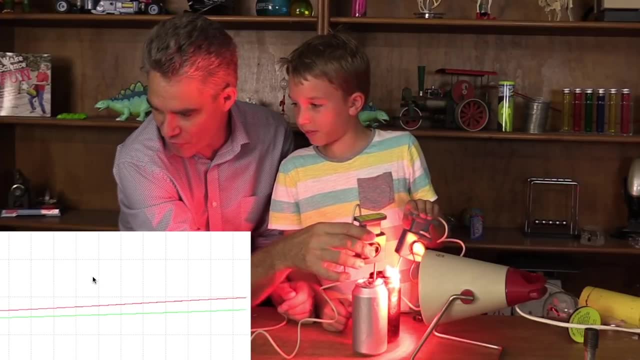 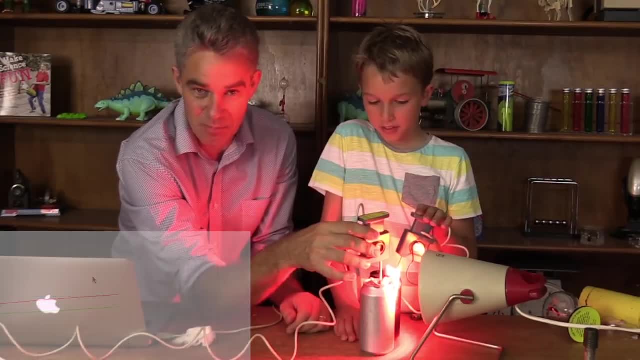 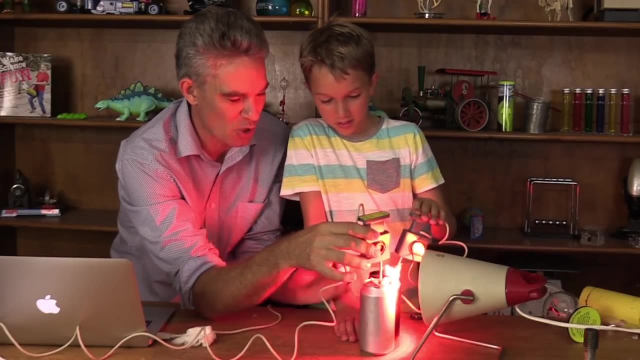 So your temperature's much higher already. That's the black can, And I can see a bit of smoke coming out of mine. Is that right? You can actually see some smoke coming out. That's how much hotter it is, Isn't that interesting?